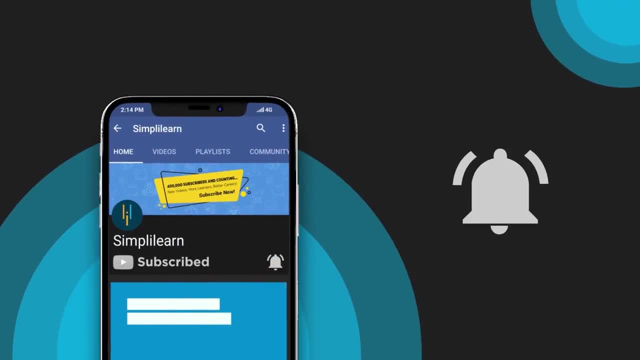 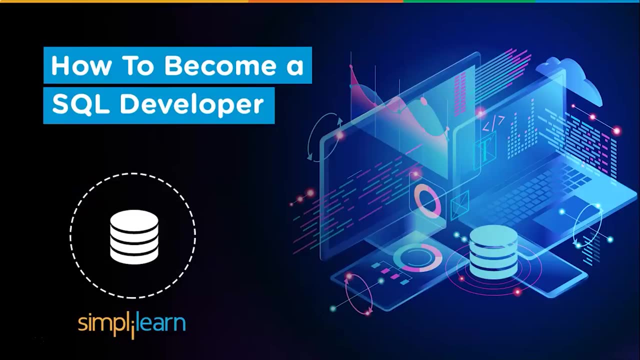 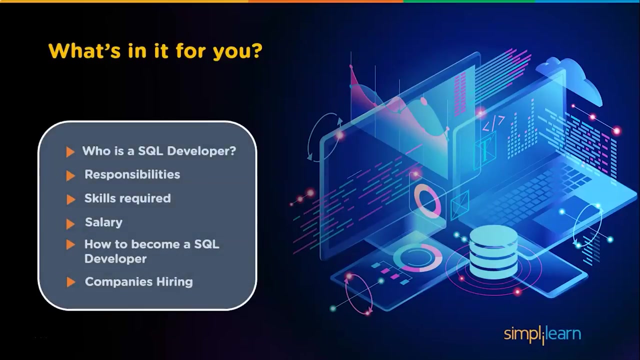 Hello everyone, welcome to this video tutorial on how to become a SQL developer by SimpliLearn. In this session we will learn who is a SQL developer and what are the responsibilities in a company. Then we will focus on the skills required to become a successful SQL developer. 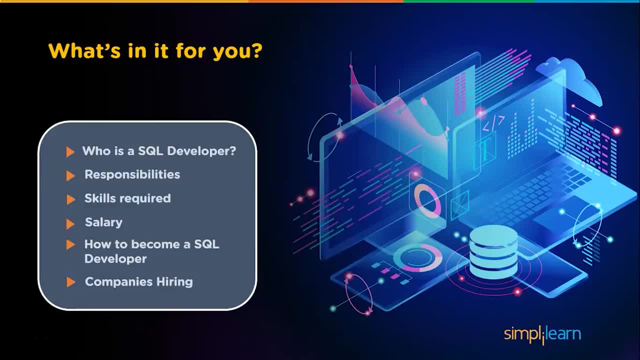 We will see the expected average salary in both US and India. We will also discuss how to become a SQL developer and look at the top companies hiring for SQL developers. So hey, everyone, I am Abhisar Ahuja from SimpliLearn, and welcome to this video on how to become. 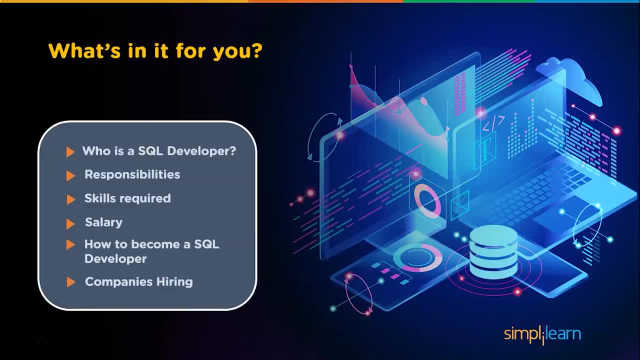 a SQL developer. But before we begin, if you love watching tech videos, subscribe to our channel and hit the bell icon to never miss an update. When going through some of the popular job boards online, you would easily see SQL developer is one of the most demanding jobs seeked by companies, As we all know today. 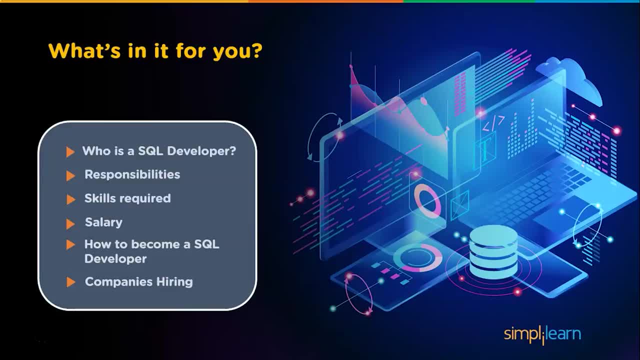 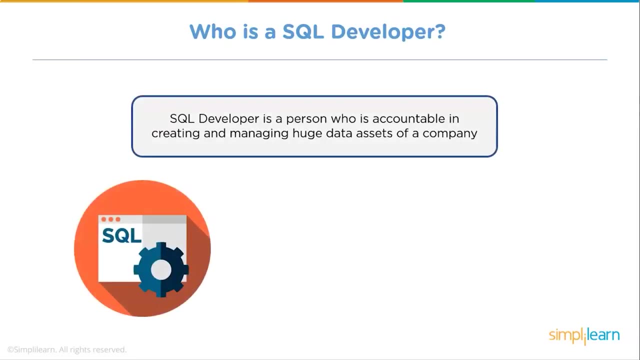 companies collect vast volumes of data and store it in their own databases. They want professionals with a good understanding of data who can keep it safe and secure. So first we will understand who is a SQL developer. SQL developer is a person who is accountable in creating and managing huge data assets of a company. 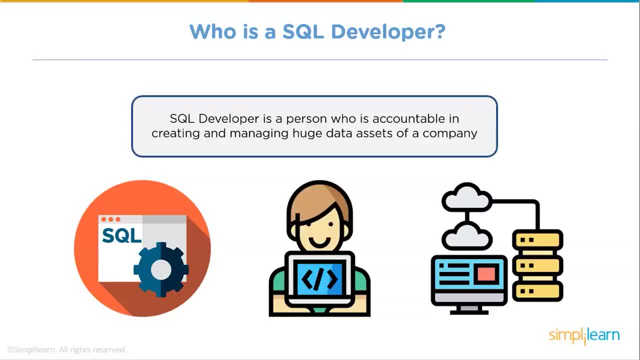 SQL developer is a person who can develop SQL databases as well as write and test code. Let's understand this with the help of an example. Let's say we want to search a particular product on the Amazon website and Amazon has stored all its data about products in. 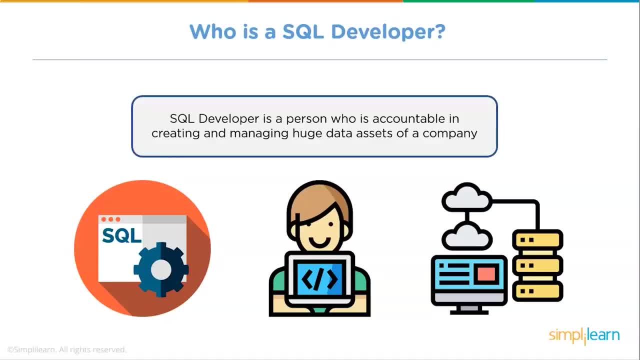 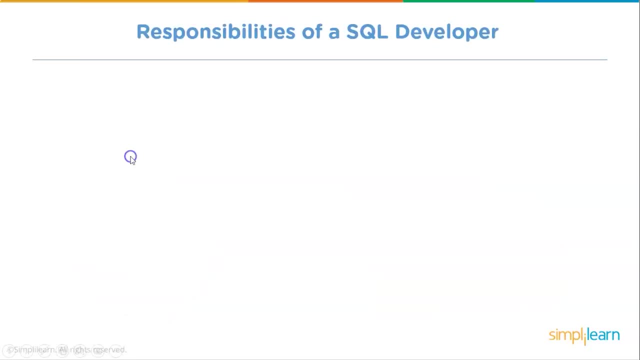 a database. Now we will write the product name in the search bar and when we click on the search button it will run a SQL query that fetches all the information about the product and displays us on the website website. So this is the basic task done by a SQL developer. 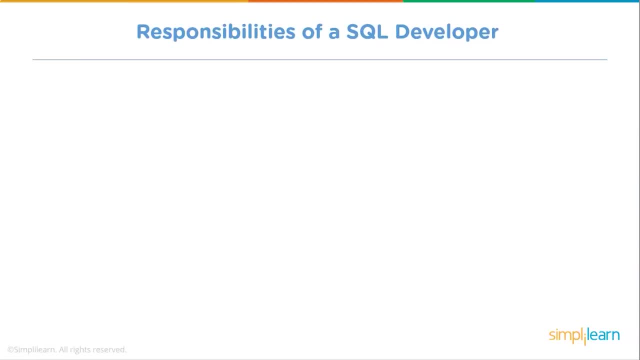 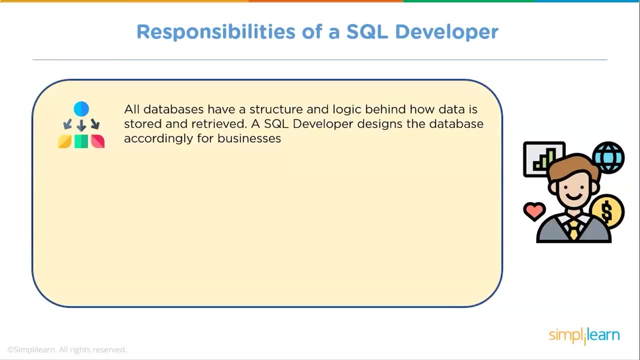 Now we will understand the responsibilities of a SQL developer. All databases have a structure and logic behind how data is stored and retrieved. A SQL developer designs the database accordingly. for businesses that is called database modeling. After the database is created and deployed, it's the SQL developer who is responsible. 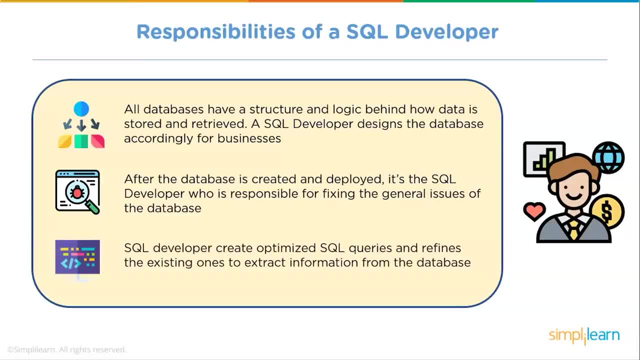 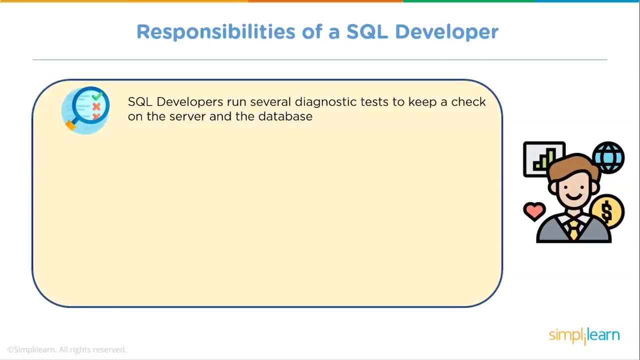 for fixing the general issues of the database. SQL developer should be well-versed with structured query language to create optimized SQL queries and refines the existing ones. to extract information from the database. SQL developers run several diagnostic tests to keep a check on the server and the database. 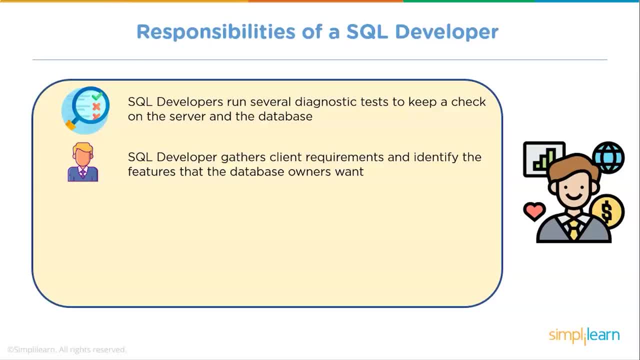 In order to understand how to organize company's data, SQL developers must communicate with tactical and non-technical persons from the business, and SQL developer also gathers client requirements and identifies the features that the database owners want. As data is an asset to a company, SQL developers backup and restore data for their clients. 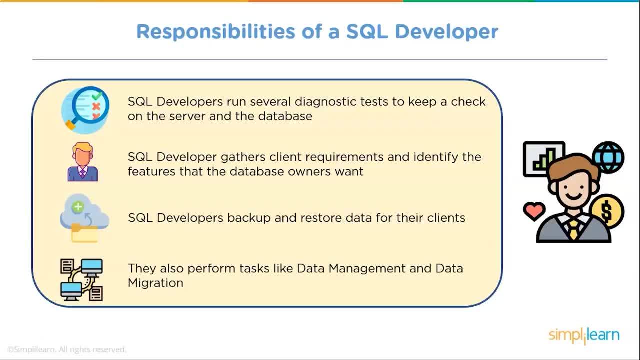 They also perform tasks like data management and data migration. That is, if a company has stored all its data on a local storage and now it wants its data to be stored in a cloud storage, so the safe transmission of the data from local storage to cloud storage is known as data migration. 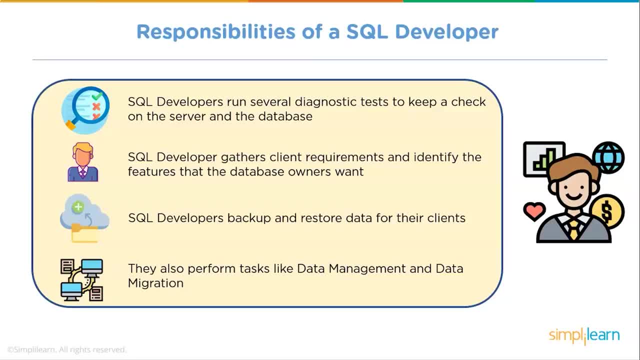 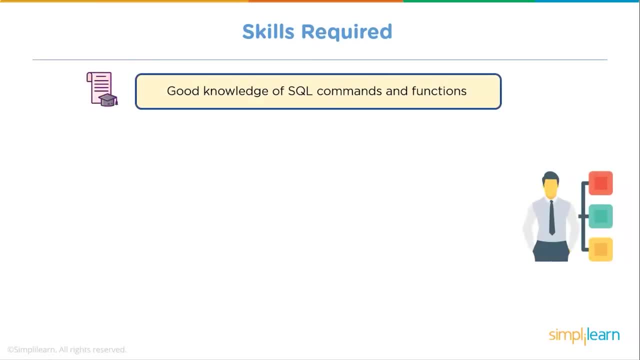 And that is done by the SQL developer. After knowing the responsibilities, now we should look for skill set required to be a good SQL developer. One should have a good knowledge of SQL commands, functions, joints and procedures. Let's have a look at few commands, such as create, drop, alter and truncate. 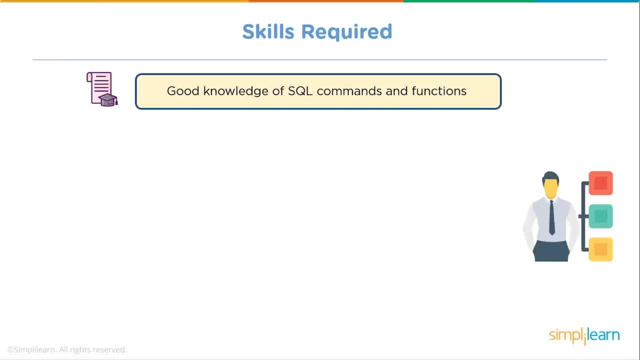 These commands come under data definition language. We also have insert, update and delete commands. These commands come under data manipulation language. We have grant and revoke commands. These commands come under data manipulation language. We have a few commands. We also have commit, rollback and save point commands. 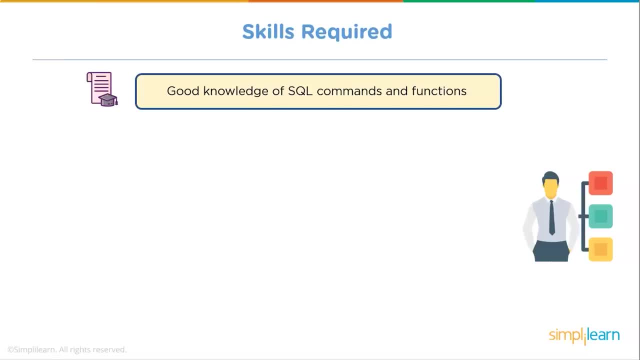 These come under transaction control language. These are the basic commands a SQL developer should be familiar with, And a SQL developer may have a little command on any one programming language. You don't have to be expert in programming. all you need is how to interface between application. 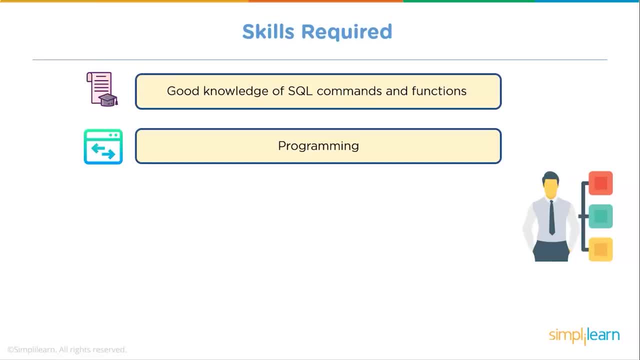 and your database. For example, you are using MySQL and your web application is based on PHP, then you should know how to connect your application to the database and how to issue queries, how to fetch results and then how to display it to the users. 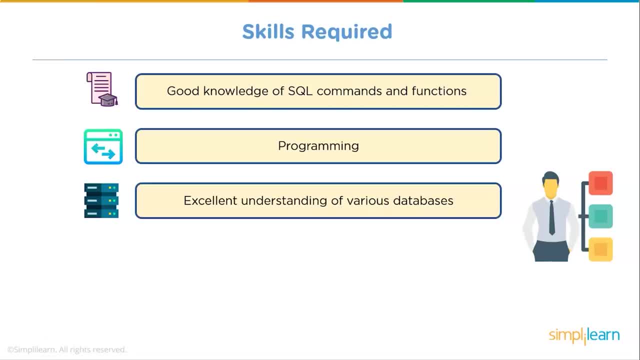 One should have a good understanding of various database management systems such as MySQL, Microsoft Access, Oracle, PostgreSQL Dbase, FoxPro, SQLite, IBM DB2, LibreOffice Base, MariaDB and Microsoft SQL Server. One should know integration of databases with data visualization software such as PowerBI. 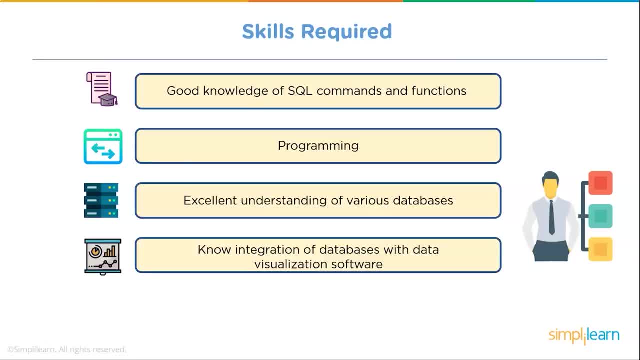 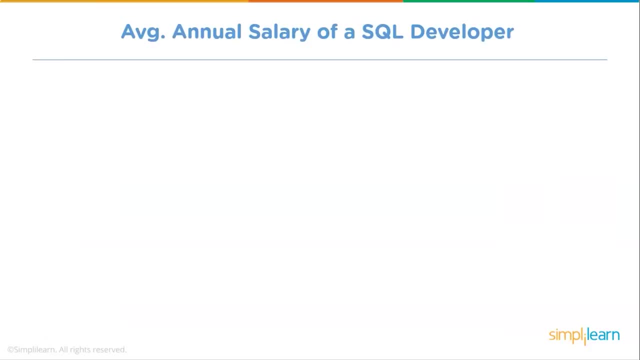 and Tableau, which helps businesses to make better decisions and give you an add-on. as a SQL developer, One should develop critical thinking and problem solving skills to create optimized queries. Now we will see how a SQL developer is compensated in both United States and India. 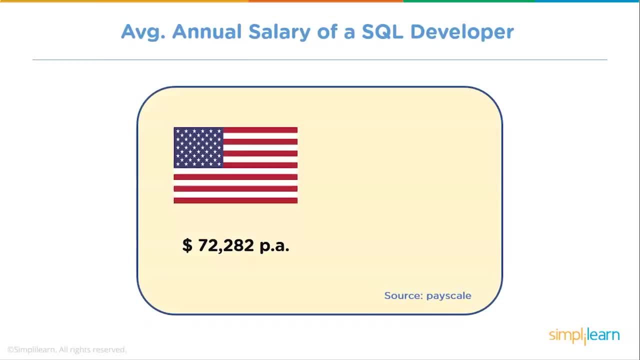 In the United States, SQL developers draw an average salary of $10 per month. In India, the average salary of a SQL developer is ₹ 4,49,532.. Now we will see how a person can become a good SQL developer. For that, one should have a good command on structured query language and know how to. 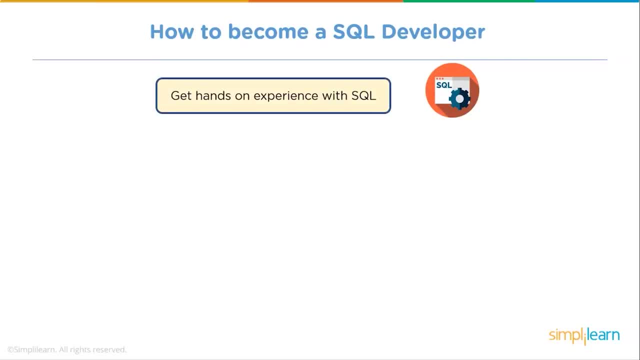 interact with database management system and can issue queries to get the desired result, Earning industry-recognized SQL developer certifications. one should have a good understanding of the database capabilities and knowledge on Preparation, Determination And лежing experience. So the best example of this is being a SQL developer who can work in a business. 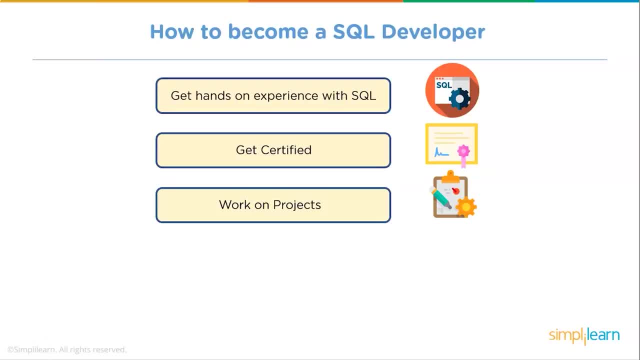 In India, one can get a good amount of money for its work. In India, one can get a good amount of money for its work. So one can get a good amount of money for its work. That's all the ways to work as a designer. And one can get a good amount of money for its work. So here is the list of the best services for the people with the ability to develop SQL developer. Click the link in the description. In the description I will mention all the dells I use, and this is a very important example. 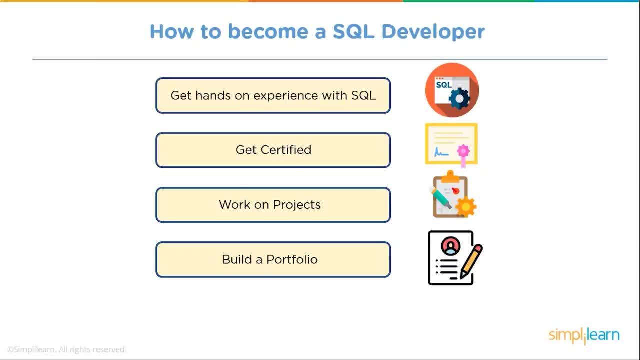 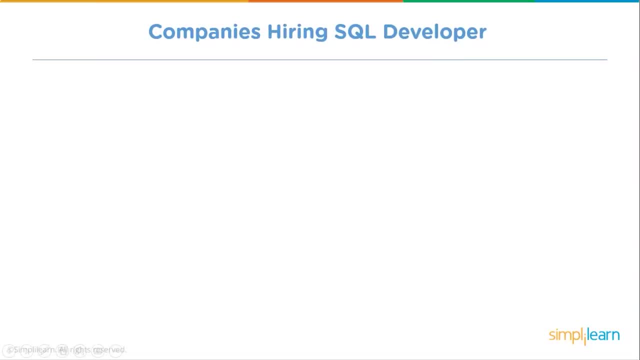 You can check the links in the description. Check the links in the description as well. If you find any nice examples regarding SQL developer, you can do so now: experience, test your knowledge and build your project portfolio, which will be highly beneficial when you start applying for your first full-time position.